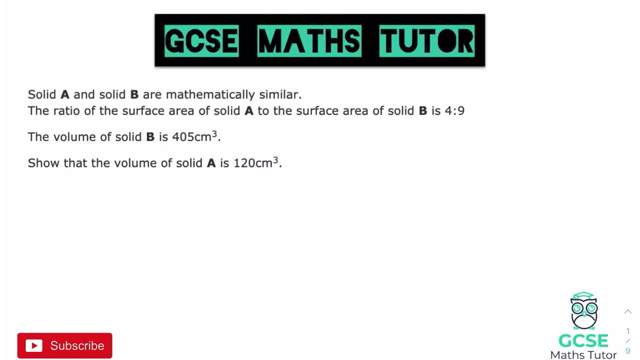 sec. It says the ratio of the surface area of solid A to the surface area of solid B is 4 to 9, and then it says the volume of solid B is 405,. show that the volume of solid A is 120. Now obviously we've got the ratio involved here. it gives us the ratio of their. 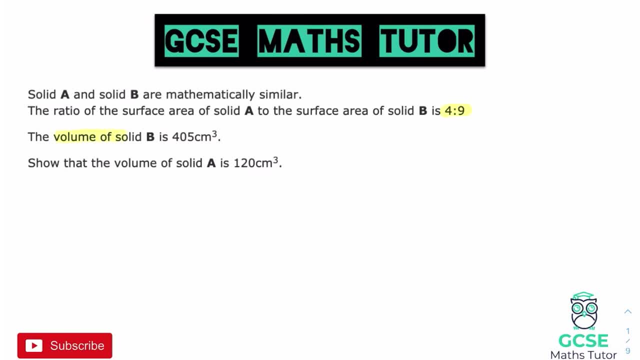 surface areas. It then asks us to look at the volume of those shapes. okay, and it gives us the volume of solid B, and it wants us to show that the volume of solid B is 120, and it wants us to show that the volume of solid B is 120, and it wants us to show that. 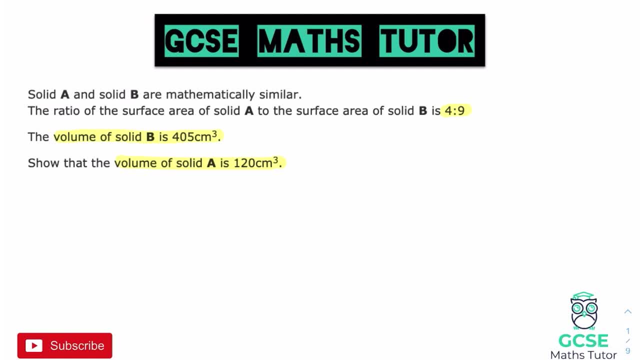 the volume of solid A is 120.. So if we actually have a look at this and thinking about how we would do this in a non-calculator method, we need to move between the surface area ratio up to the volume ratio. Now we have a look at this and if we label this, we've got the 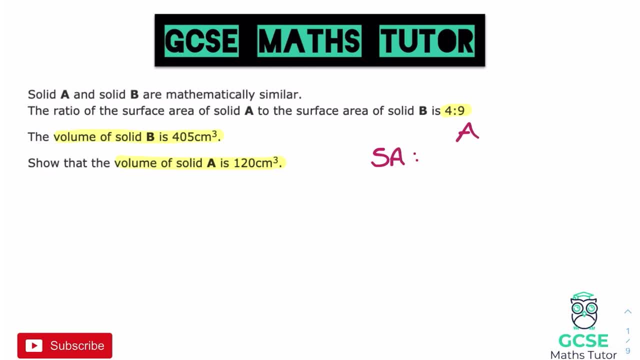 surface area and we have A and we have B, and at the moment that's in the ratio 4 to 9.. Now, to get from surface area back to the volume, which is what we're looking for here, we're going to have to first go back to the length. 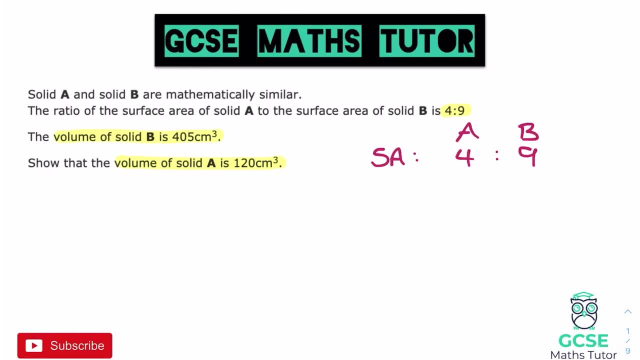 So, in order to get from our surface area to our length, we need to square root it, okay, and that's how we move between our similar shape ratios here. So to start with, we're going to go to the length, okay, so I'm just going to write that down as L and to get 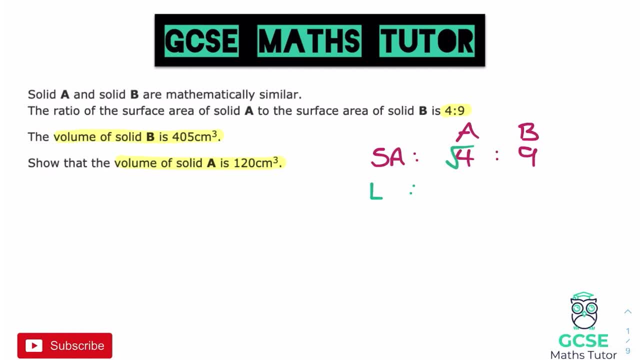 there we're going to square root both those numbers, so the square root of 4 and the square root of 9, that gives us 2 to 3.. So our length ratio here is 2 to 3.. Now, from there we're. 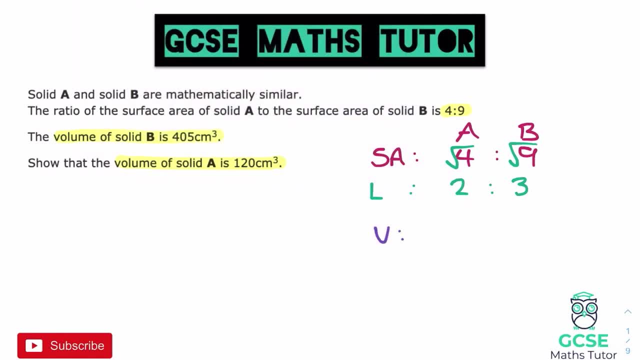 going to want to get to the volume. Now I'm just going to label this volume and to get from length to volume, we need to cube those numbers. So to get our ratio here for the volume, we're going to cube them both. So we're going to cube 2, and we're going to 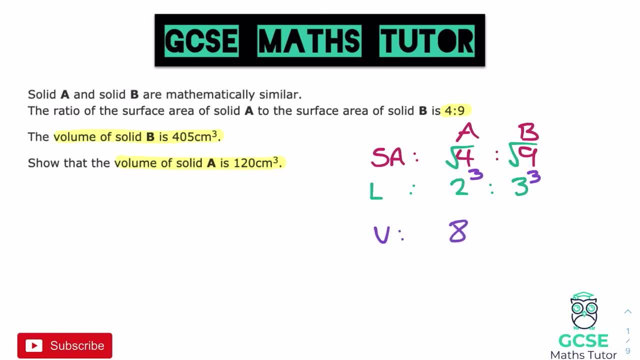 cube 3.. Now, the cube of 2 is 8, and the cube of 3 is 27.. So, in order to look at the ratio of their volumes, we're going to need to use the ratio 8 to 27.. Now, obviously, what I'm 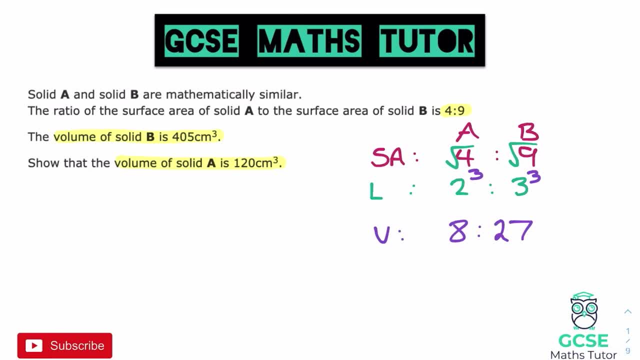 looking at. here is a non-calculator method and we will discuss that in a bit, but I'm going to use a calculator method as well. but I think this is quite a nice non-calculator question. So let's have a look Now. it says that the volume of B is 405 and the volume 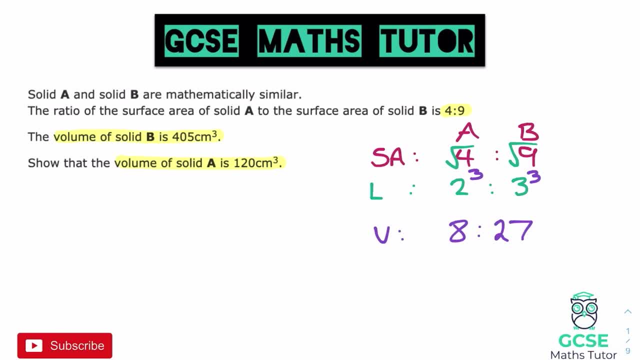 of A is 120.. Now obviously we can tell just by looking at those that A is the smaller shape here, which we can also tell from their surface areas, as it has that number 4 rather than the 9.. But if we were to draw a little picture here, we can imagine a smaller shape. 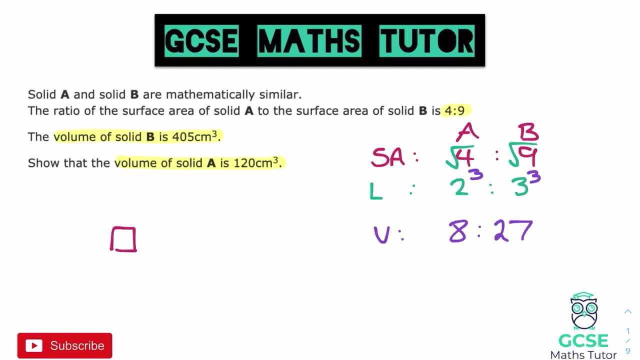 obviously I'm drawing a 2D shape here, but it's a 3D shape if we're looking at volume and we have the larger shape. So we've got this one as A and this one as B. Now at the moment it says the volume. 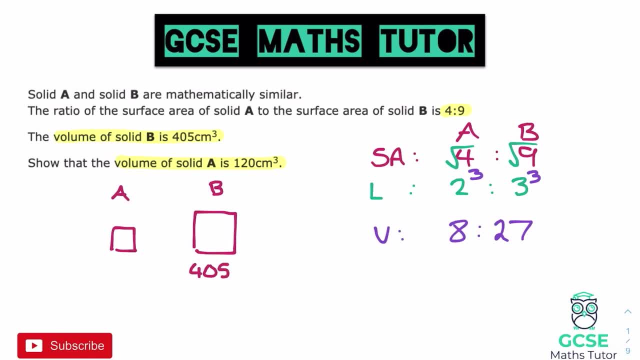 of solid B is 405, so let's label that 405 centimetre cubed. And if we align that with our ratio, which we've got over here- 8 to 27,. the 405 there is below the 27.. And what? 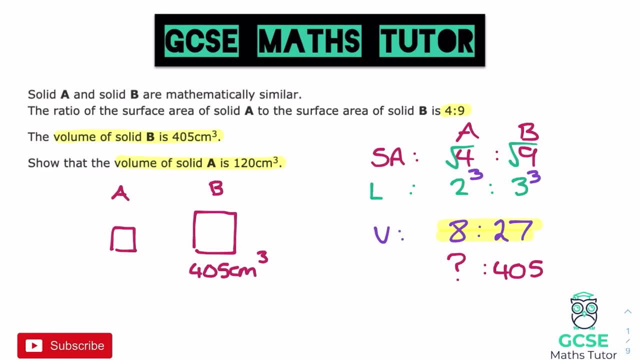 we're trying to find is what this number is that would go under the 8.. Obviously, it's told us that number, but the language there says show that the volume is 20. So we're actually going to have to show our working out in order to show that it's definitely. 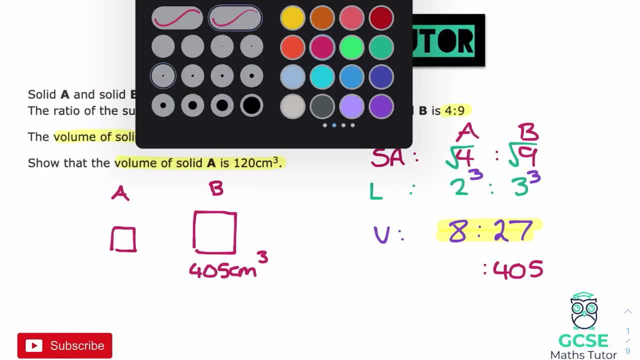 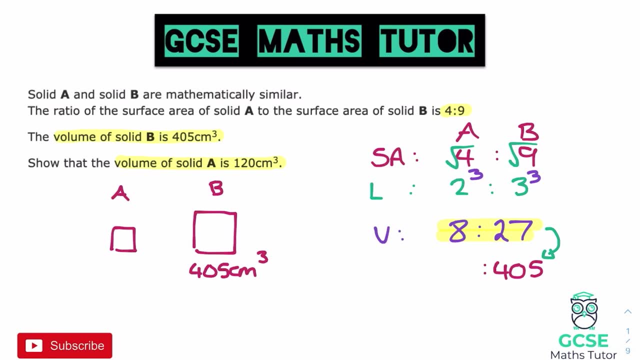 120.. Now, looking at that, all we need to think about is how do we get from 27 to 405, or in other words, what have we multiplied by to get there? And in order to figure that out, we need to do 405 divided by 27.. Now, obviously you can use some bus stop for that. 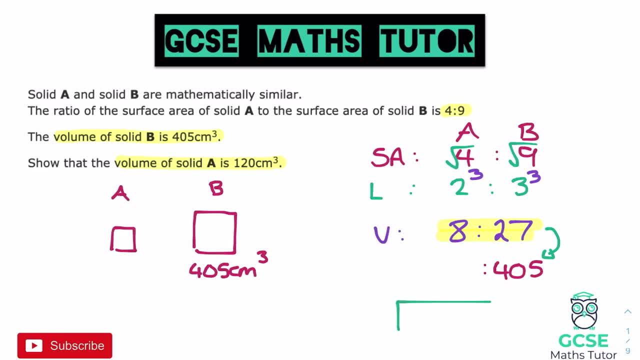 obviously, if it's non-calculated. If we have a calculator for this, it's nice and easy, but this can actually be the non-calculator. So let's see how many 27s go into 405.. Now, 27 goes into 40 once and there'll be a remainder there of 13,. so that's going to take us up. 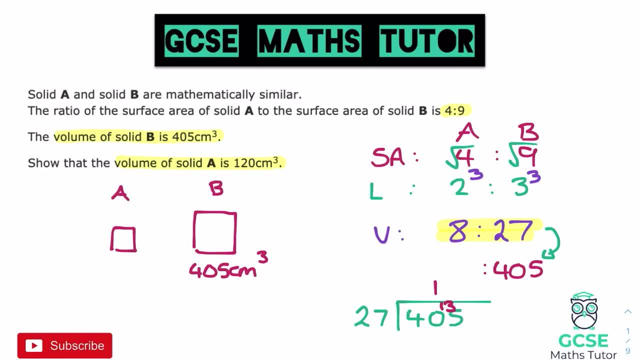 to 135 for the next one. How many times does 27 go into 135? Not the nicest. there We could write out some of the 27 times table, but actually it ends in a five and that gives us a bit of a hint that it is five. Always check that, But it is actually 15 times there. 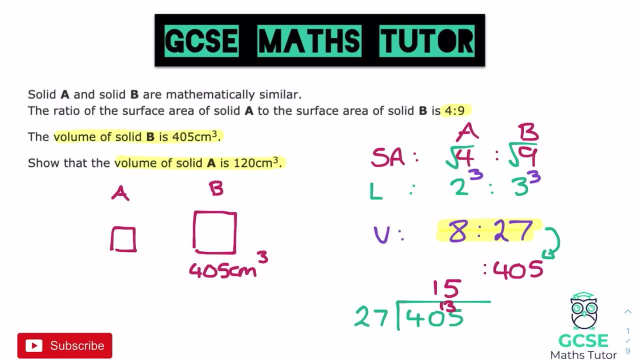 and it's five times that 27 goes into 135. So that means we've multiplied by 15. in this ratio that 8, that part of the volume down to our actual volume, here we need to times by 15.. 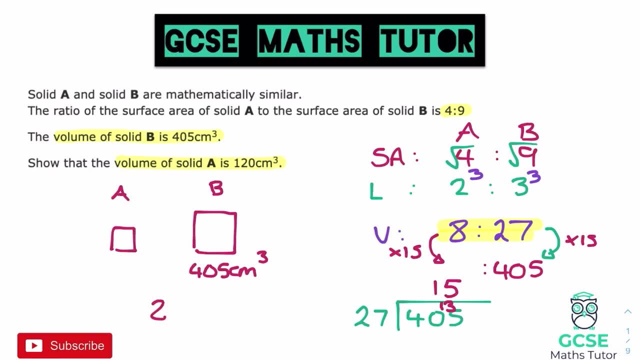 And 8 times 15, again we could show that on the working out, 8 times 15 gives us an answer of 120.. And there we go. We've shown there that the volume is going to be 120 centimetre. 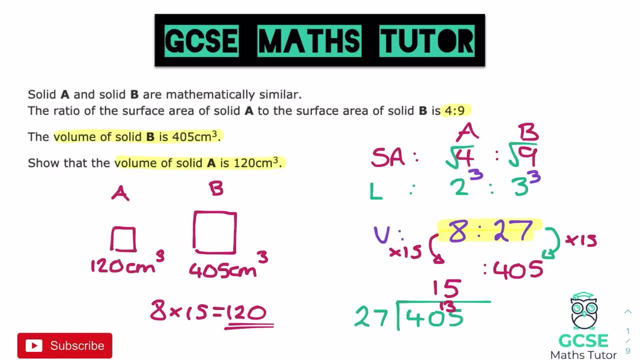 cubed, And that's enough to show you're working out. there. We've shown that we've moved between the ratios there from surface area to length and then from length to volume, And then we've shown within that volume ratio how we got from 27 to 405, and therefore replicating. 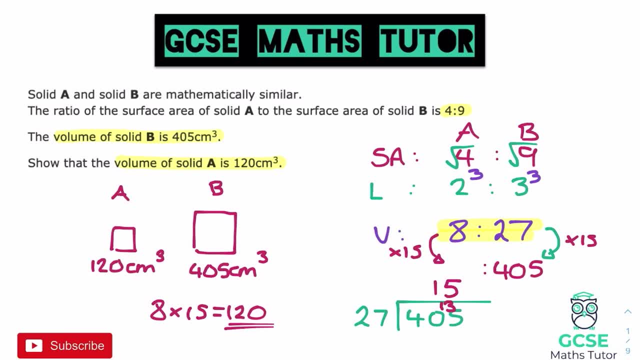 that with the 8.. Now, that's one method that you could use non-calculator. There is actually a calculator method that we could use here as well- although this particular question was a non-calculator question- with some quite nasty little divisions and multiplications. 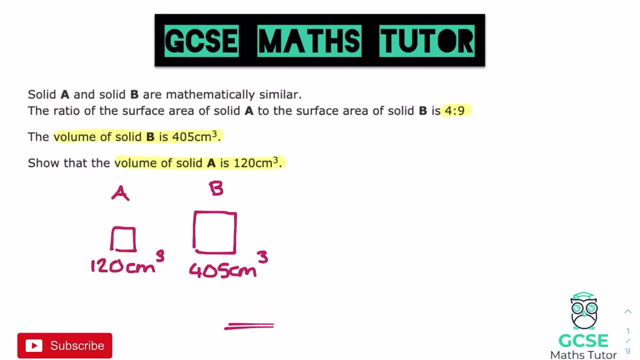 in there. But let's have a look here at a calculator method. Now again, this is what we're trying to show- that we get from 405 to 120.. Now what you can do is you can just take this ratio and just like normal with similar shapes. you can take this ratio and 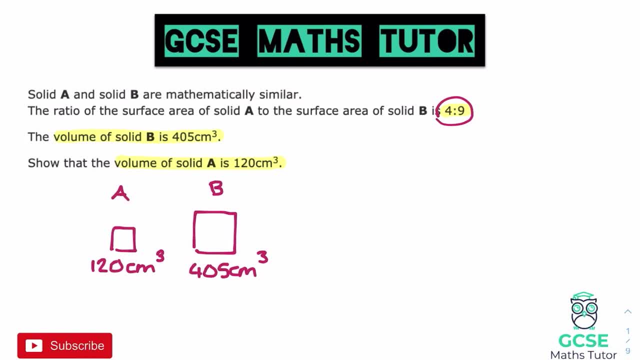 do the big number divided by the little one, So 9 divided by 4.. And we're going to do this on the calculator, so I'm going to type that in 9 divided by 4 gives us 2.25.. So 2.25,. 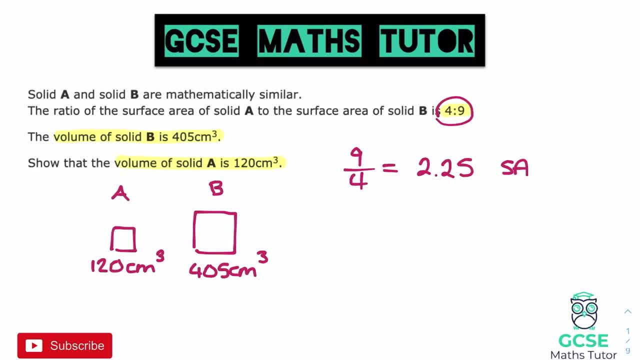 and that is our surface area scale factor. Okay, so we're looking at a scale factor now. Now again, to move from surface area up to volume, we're going to have to first figure out our length. So again, same process: We're going to square root that. 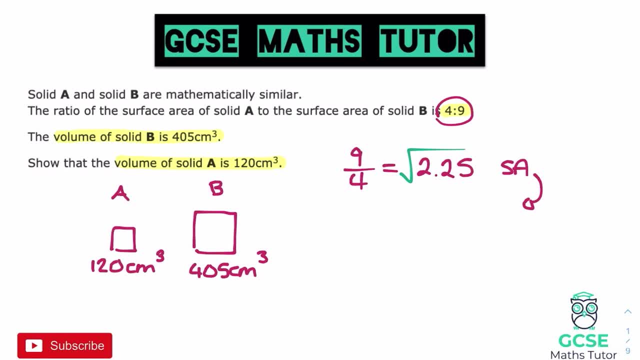 And if we square root that which again I'm going to do on the calculator, we get 1.5.. So 1.5, and that is our length scale factor. Now we want to get from length back to volume. So you can see, it's a very similar process, It's always the same way, moving between them. 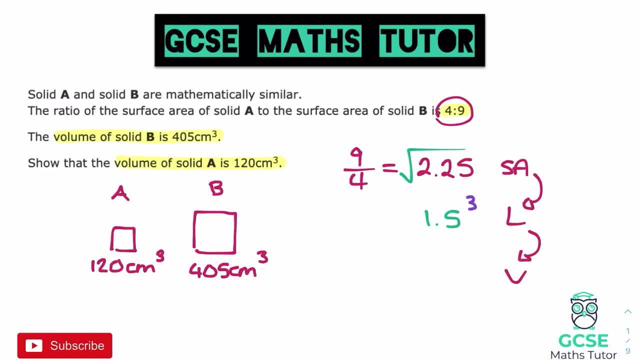 But we're going to have to cube 1.5.. So again, I'm just going to do that on the calculator: 1.5 cubed and that gives me 3.375.. And that's my volume scale factor Now in order to use. 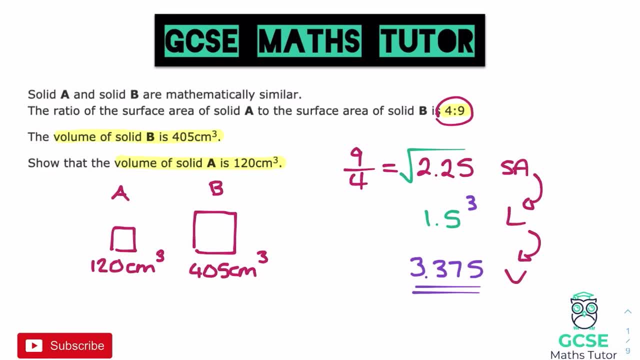 that all I need to do is I need to look at which one I have And in this case we have the bigger volume And if we're going down to the smaller one we need to divide by that scale factor, So divide by 3.375.. And let's just check that on the calculator: 405 divided. 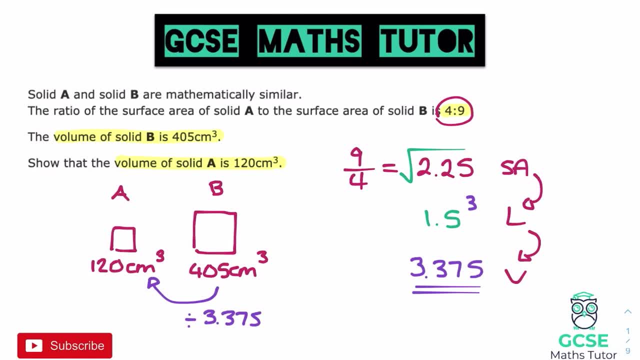 by 3.375, and that in fact does give us 120.. Obviously, we're doing this on the calculator, so we don't need to show our working out for that, But we do need to show here what we've actually done. We've divided by 3.375, and obviously just confirming that gives us the. 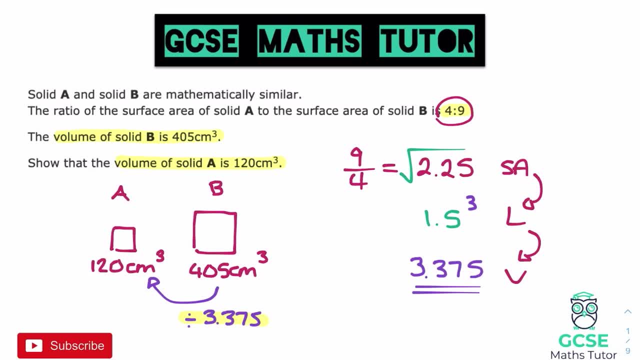 right answer, So we can do that either way. Up to you which method you choose, if you have a calculator or if it's a calculator question. Obviously, if it's non-calculator- though, it's more than likely- you're going to have to use that method that I used previously, And actually that 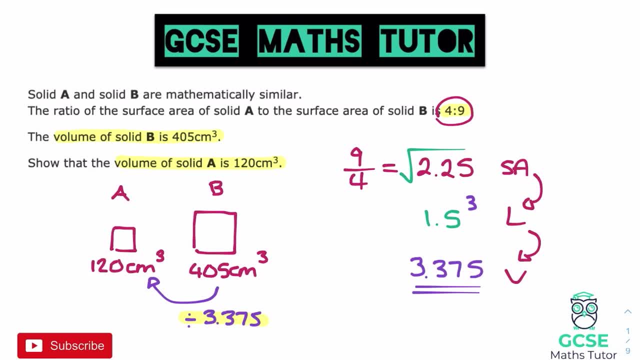 method can be used, or this method that I've just done can be used non-calculator as well. Obviously, just as long as this number here comes out as a whole number, We wouldn't really be expected to square root 2.25 and cube it without a calculator. But that is another. 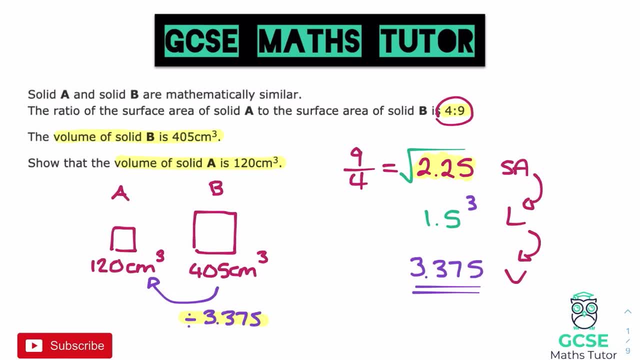 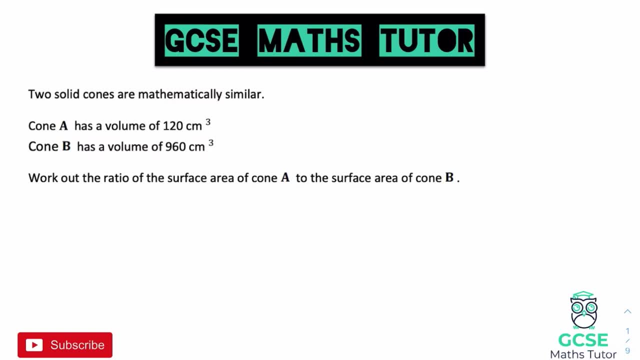 method that can be used, even if it is non-calculator, just depending on the numbers there. But there we go. there's an example of one of these questions. Let's have a look at another one. Okay, so we have a very similar styled question here for our second question. It says two. 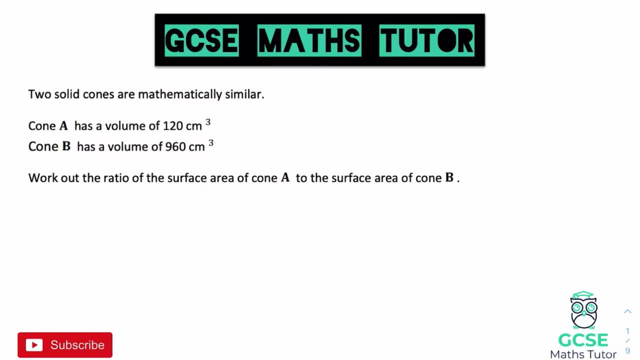 solid cones are mathematically similar. Cone A has a volume of 120, and Cone B has a volume of 960.. Work out the ratio of the surface area of Cone A to the surface area of Cone B. Now, in order to work out a ratio here, all we really need to do is get the ratio. of the surface area of Cone A to the surface area of Cone B. Now, in order to work out a ratio here, all we really need to do is get the ratio of the surface area of Cone B to the surface area of Cone B Now in order to work out a ratio here, all we really need 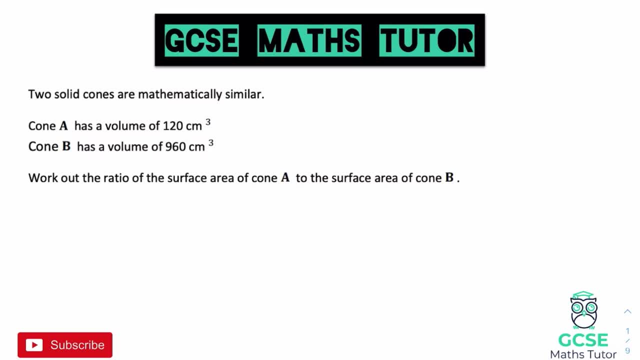 to do is get the ratio of the surface area of Cone B to the surface area of Cone B, And what we need to figure out is how much bigger one is than the other. And again, we're going to take this approach as a non-calculator method to start with And, in fact, our method. 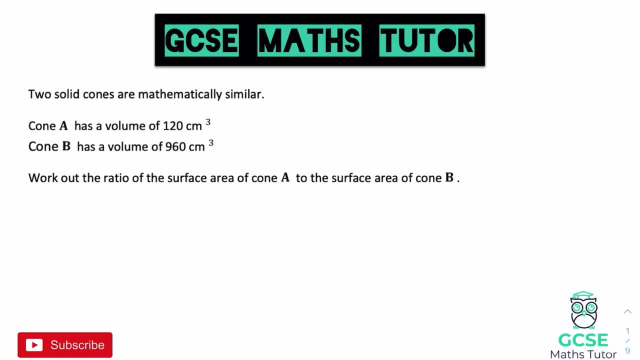 that I'm actually going to use here is going to be very similar, even if we were using a calculator Now to figure out the volume scale factor. as we've been given the volume of both of these, I'm going to take the big one and divide it by the little one, just like I did on the 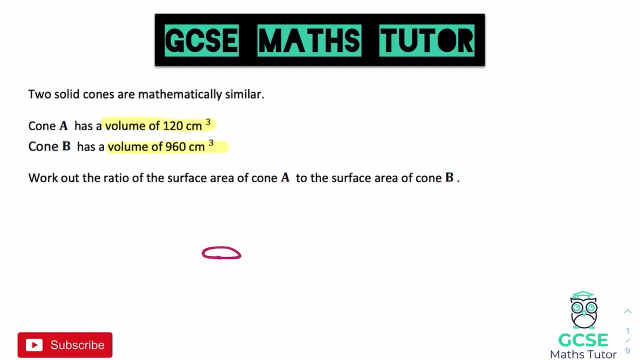 last question with the ratios. So I'm just going to draw a little diagram here just so we can kind of visualise this a bit, As we have Cone A, which is our smaller cone, and Cone B there, which is our larger cone. So if we take the bigger one and divide it by 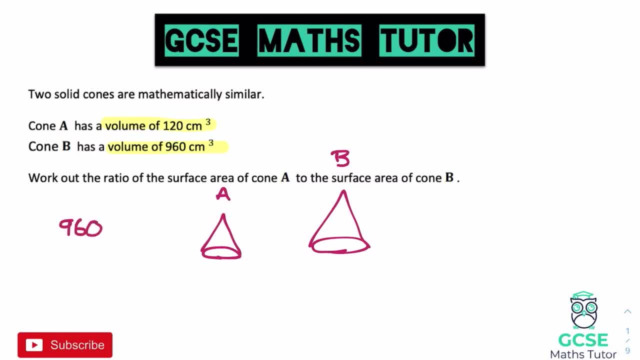 the smaller one. we're going to do 960 divided by 120.. And again, if you didn't have a calculator right now, you could do 96 divided by 12 and just take your time with that, But that comes out as 8.. So if we think about what we've got here, we have our volume scale factor. 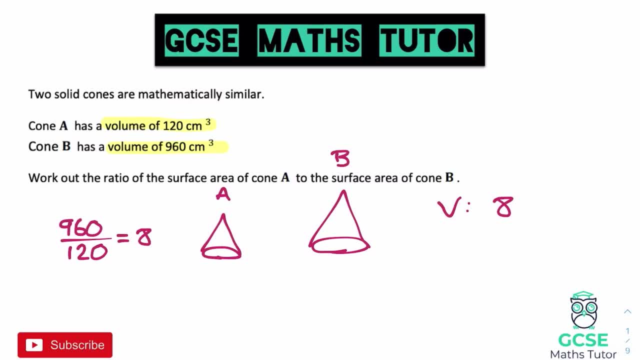 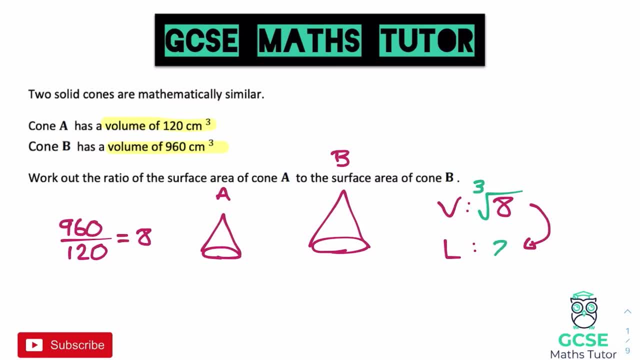 and the cube root of 8 should be able to be done without a calculator. The answer there is 2.. It's 2 times 2 times 2.. From length we can get back to area, as we're being asked about an area scale factor here. 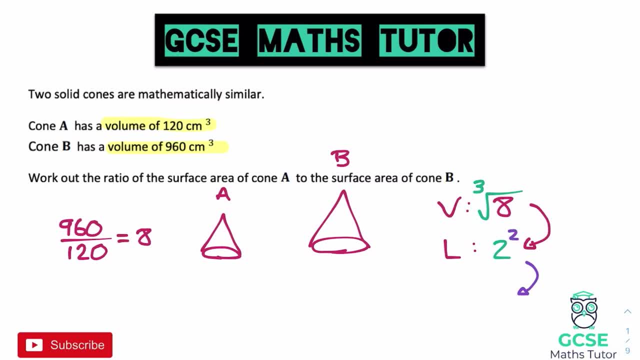 And to get from area, from length, we're going to square that, just like we did before when we square-rooted in the other direction. Now, 2 squared is 4.. So, in other words, our scale factor in terms of the lengths is 4.. 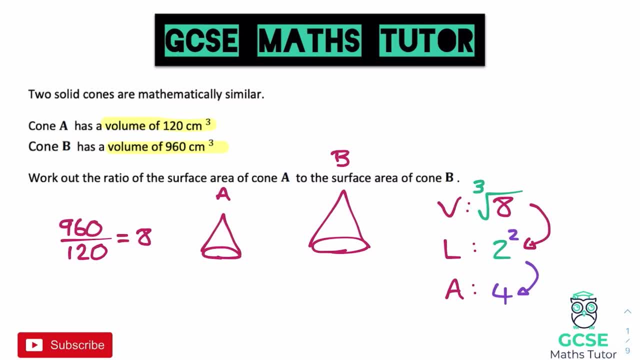 Now, a scale factor of 4 means that one is 4 bigger than the other. So, in terms of writing this as a ratio, if cone A was 1, cone B would be 4. And that is our surface area ratio. 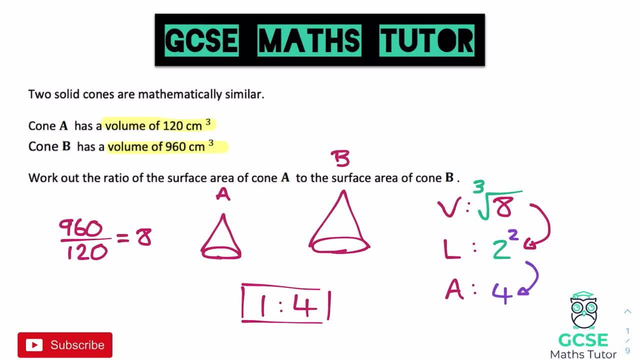 And we could have done this ratio with any of them. When it comes to the length, it would have been 1 to 2, as our scale factor there was 2 for the length. And when it came to the volume, our ratio there in terms of that scale factor would have been 1 to 8.. 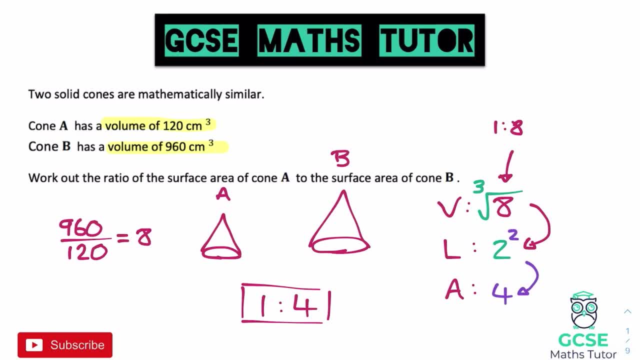 So in terms of their lengths, the lengths are twice the size that B is to A. The areas are 4 times the size from A to B And the volume is 8 times the size, again, going from A to B. 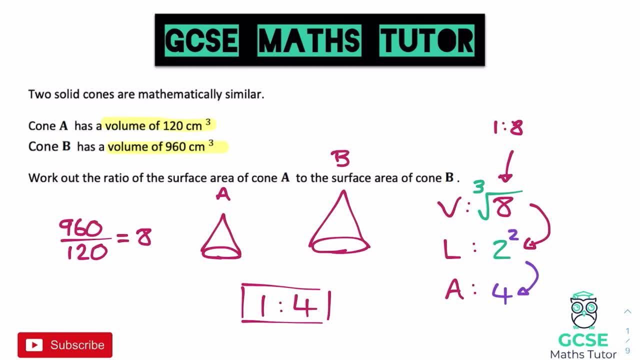 So that's how we're going to approach these questions. Obviously, it's all about moving between those scale factors: to get from length to area- U squared. to get from length to volume- U cubed- And we do the reverse, going back either way. 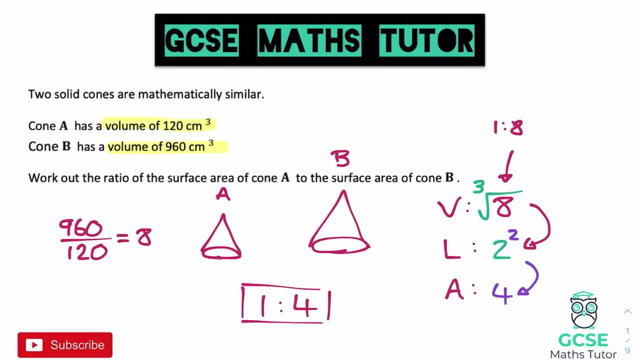 But when we're given areas and volumes we always have to go back to length, And length is our key one there, because that's like our little bridge to get between the two scale factors of area and volume. So there we go. There's another question, very similar to the last one, not as much working out there. 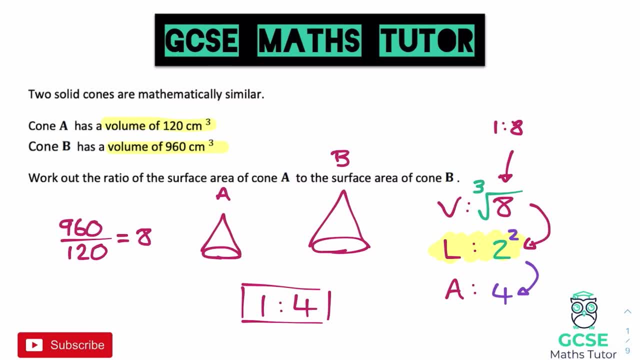 But again, just thinking about that in a slightly different way maybe, But in both scenarios there, whether we had a calculator or didn't have a calculator, we would be doing 960 divided by 120.. You could, to be fair, you could actually write these as a ratio. 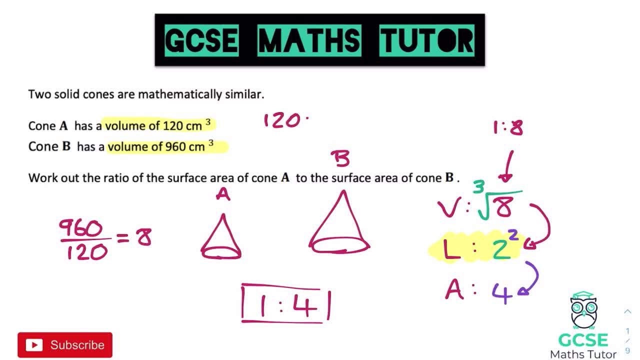 You could write that their ratios at the moment are 120 to 960 and try and simplify it from there, But ultimately you are just going to be dividing by 120 in order to get that first ratio of 1 to 8.. Okay, so it doesn't matter which method you use there. ultimately you're going to be doing the same calculation. 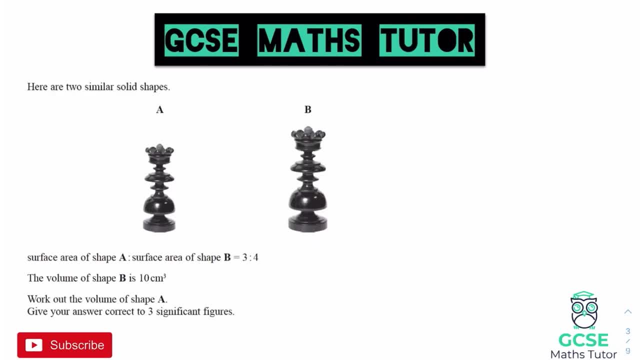 So there's our second question. Let's have a look at our final one. Okay, and so for our final question, we have something a little bit different, And this is strictly a calculator question. There is a little hint in the question that this is going to be a calculator one. 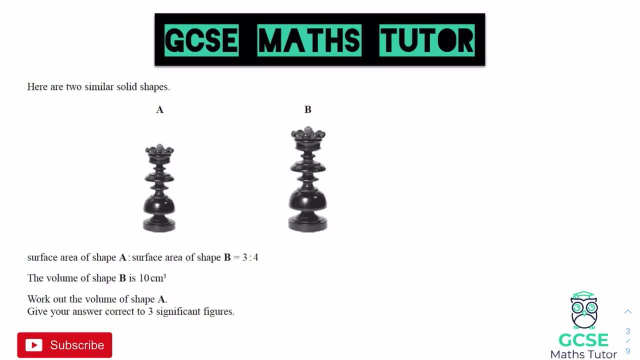 We'll have a look at that now. So it says here are two similar solid shapes and we have shape A and shape B. It says the surface area of shape A to the surface area of shape B is 3 to 4.. So it's a volume of shape B. 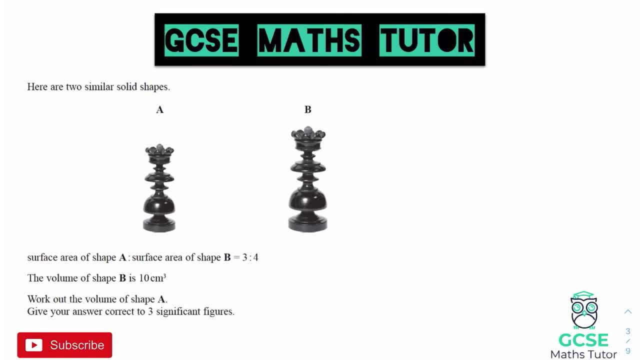 It's 10 centimetre cubed. Work out the volume of shape A. And here's our hint: that it's a calculator question. Give your answer to three significant figures. So we are only going to do this with a calculator, But again we're going to discuss two different methods. 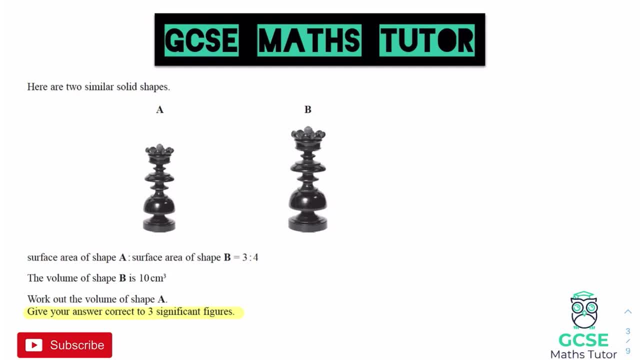 So, having a look at this, then if we take that ratio for the surface area, which we can write over here And again, let's label it like we did in the first question: We have A and we have B, And then we are going to write down our ratio. 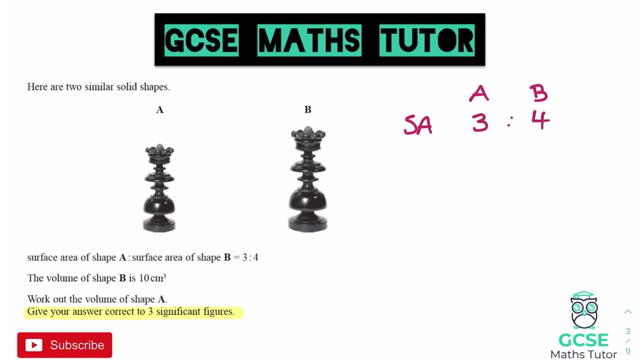 So at the moment we've got 3 to 4.. Now again, we need to get back to the first question. So to get back to length again, to get from area to length, we square root, just like we did in our first question. 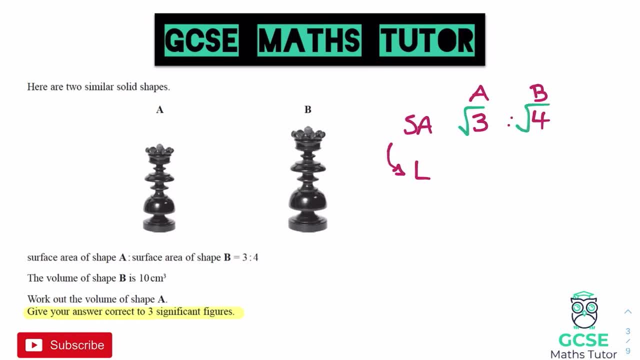 So we're going to take the square root of 3 and the square root of 4.. Now, hopefully you've spotted this isn't so nice here. The square root of 4 is OK, That's 2.. But the square root of 3, we're going to have to leave as a third. 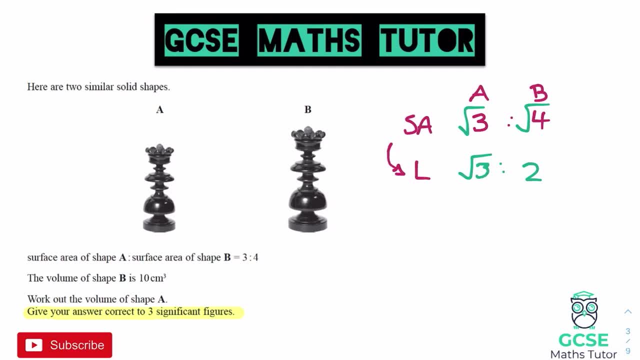 It's going to be root 3.. So we've got a little bit of trickiness going on in this question if we were to approach it in this way. Now again, we don't want length, We want to look at volume. So we're going to have to move now from length to volume. 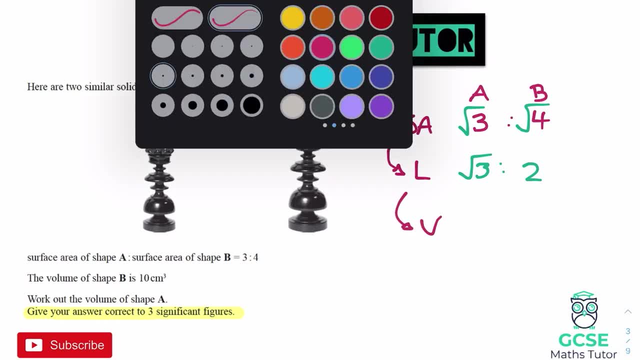 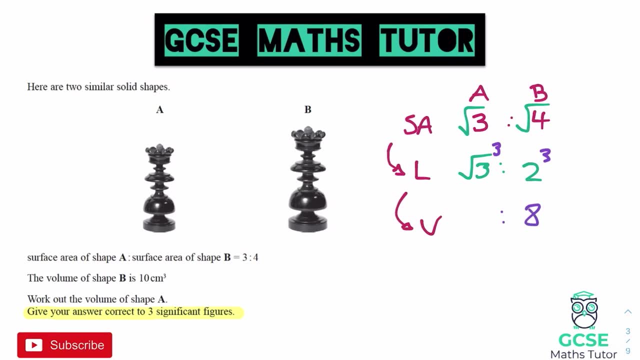 And to get from length to volume again, we already know we cube it, So we're going to cube both of these, And again we have a calculator: 2 cubed is 8.. And then we also need to cube root 3.. 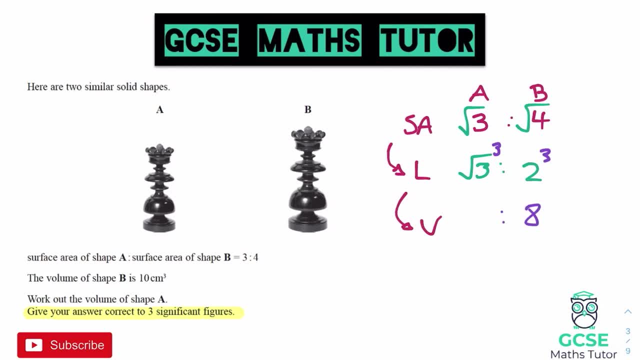 You can do that on the calculator If you know your thirds root 3 times root 3 is 3 times another root 3 is 3 root 3.. OK, And obviously if you type that into your calculator, 3 root 3 comes out as quite a nasty decimal. 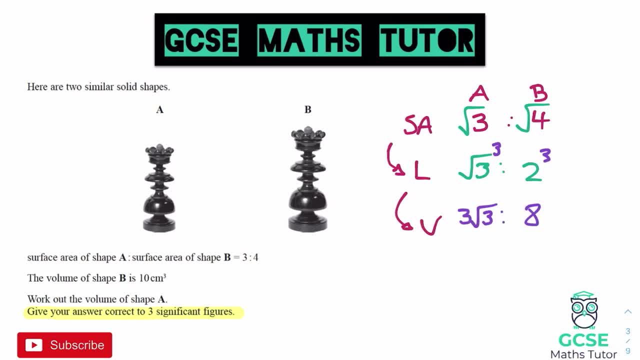 It's 5.19615.. Quite a lot of decimals there. So in terms of our volume ratio, these are our two numbers, that we have 3 root 3 to 8.. And again, if we line these up, we have shape A and we have shape B. 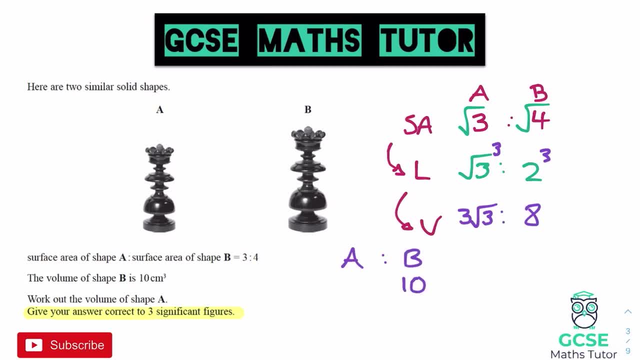 And it's given us the volume of shape B, It's 10.. Now let's just get rid of that and put our other ratio underneath there instead. So we have 3 root 3 to 8 as our ratio, And it's given us the volume of shape B. 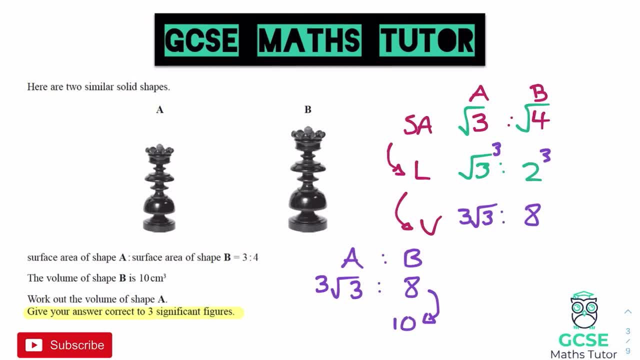 That's 10.. Now, again, just like before, We want to figure out how have we got from 8 to 10.. And we can do that by doing 10 divided by 8.. So if we do 10 divided by 8.. 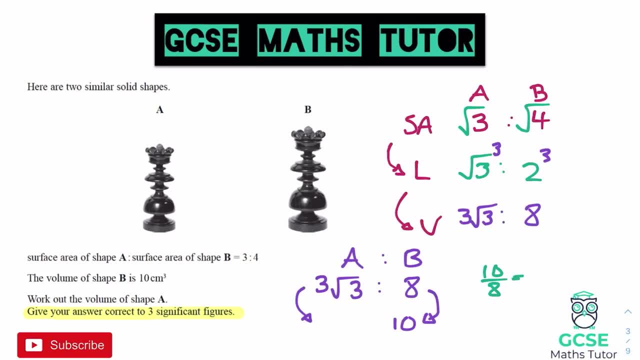 And again we have a calculator, But that obviously can be simplified to 5 over 4. Or it comes out as 1.25.. And again, just check that on your calculator, Make sure you're OK with that. So 1.25.. 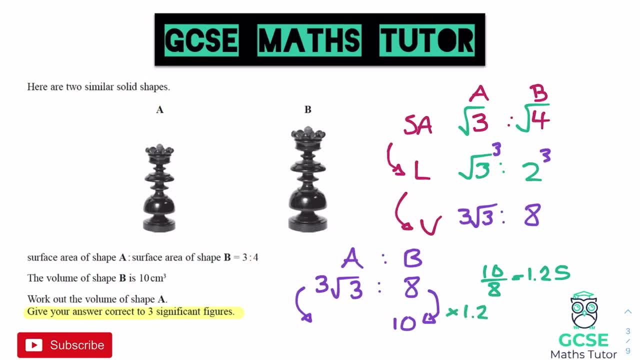 So to get from 8 to 10, we've multiplied by 1.25.. And we're just going to do the same on the other side, Times 1.. Let's get rid of that. That's not come out Very well. 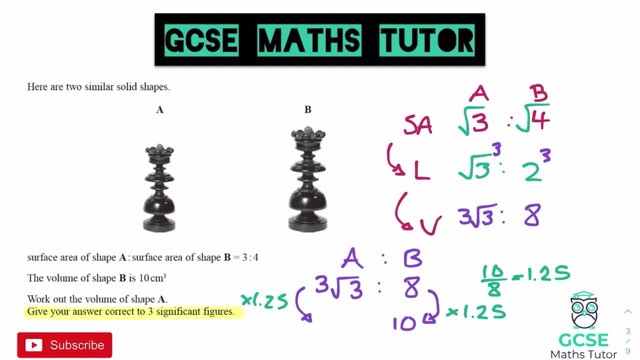 We're going to multiply by 1.25.. So on your calculator you can just do 3 root 3.. And then times that by 1.25.. And we get our answer here And it comes out as a decimal. 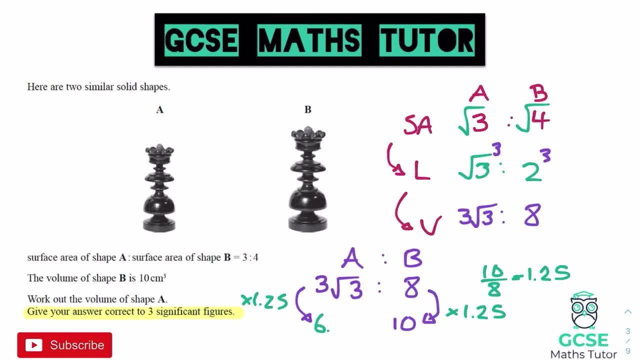 It comes out as 6.495.. And a few more decimals. I'm going to leave it there, Because obviously it wants our answer to 3 significant figures, So we can round that from there, as I've already written it out to 4 significant figures. 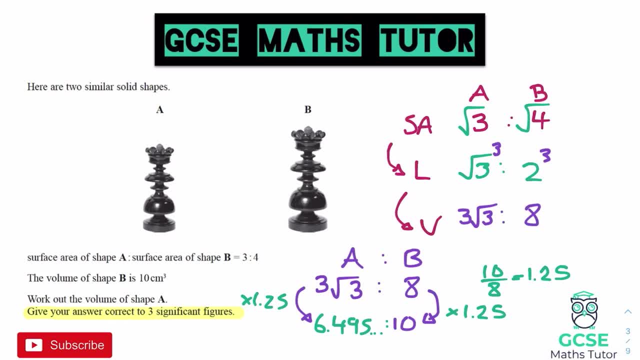 So, again, if we chop that after our 3rd significant figure- so 6,, 4,, 9,, there we go. There's a 5 afterwards, which is always a bit weird when you have to round like this, as it rounds the 9 up which rounds the 4 up before it. 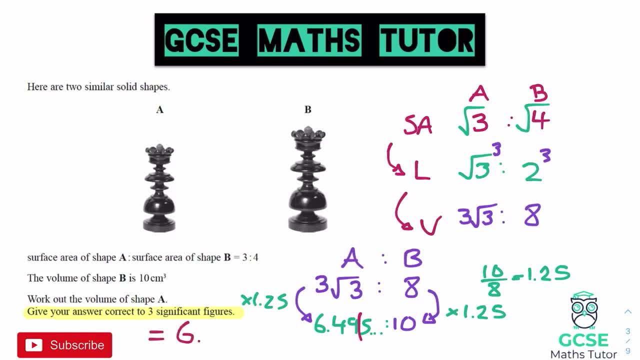 So it actually comes out as 6.5. But we have to also keep that 0 in there, as it does want it to 3 significant figures, And that 0 counts as our 3rd significant figure there. Obviously, we're looking at volume. 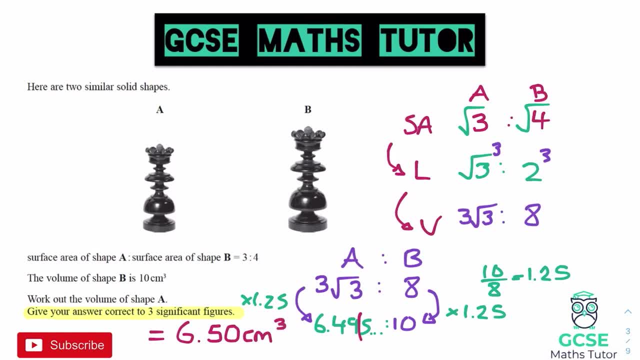 So that is centimetre cubed, Not forgetting units. But there we go. There's our final answer: 6.5 centimetre cubed. And that was only one method of doing it. Obviously, we could take another approach. 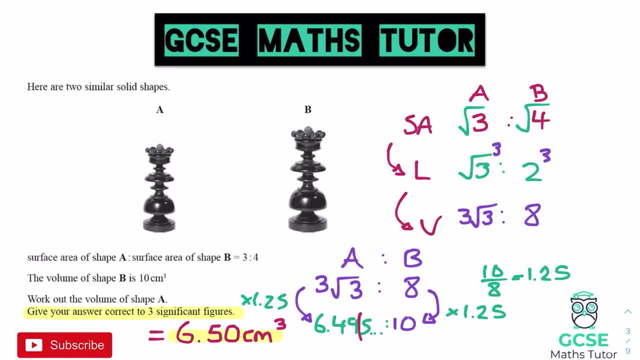 So if we get rid of this working out, we'll leave the answer of 6.5 there. But let's just have a look at our other method that we also used in question 1.. And that is taking that ratio and again doing the big number divided by the little number. 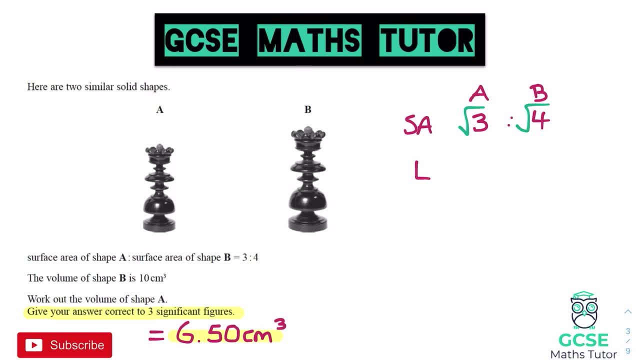 And if I keep all of this here, we'll have a look at how we move between them. So again, if I do the big number and divide it by the little number, it's 4 divided by 3.. So for our surface area, 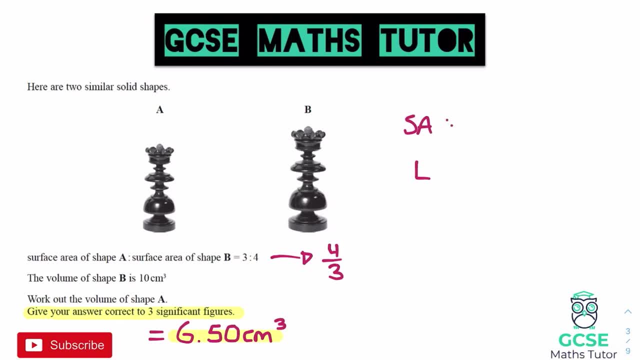 to get our scale factor, we can do 4 over 3. And that comes out as 4 thirds. So our surface area scale factor is 4 thirds Again, we can move that down to length by square rooting it. So if we do the square root of 4 thirds, 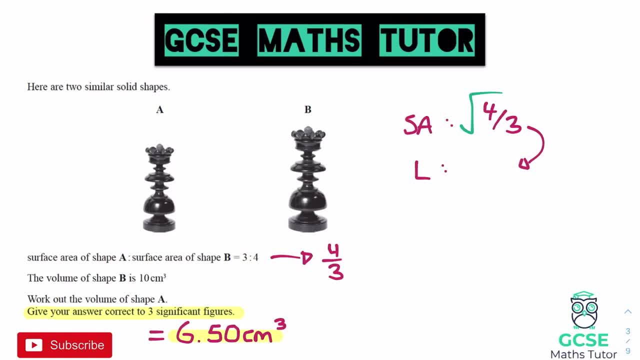 And again I'm just going to type that in on the calculator Type in 4 thirds And I'm going to do the square root of the answer And that comes out as quite a nasty number. It comes out. And again you'll see why I used the other method to start with. 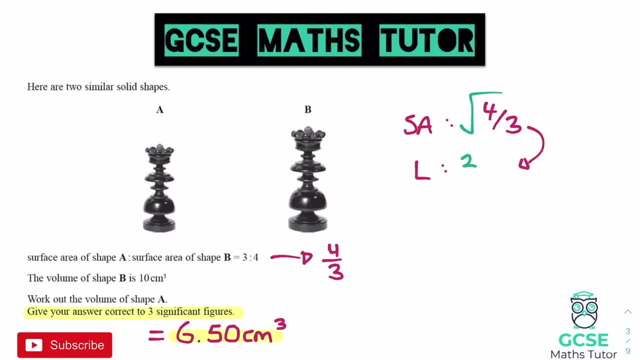 It gives us length scale factor 2 root 3 over 3.. Which is just quite a nasty decimal, 1.1547, and some more numbers there. But that is our length scale factor And again we can take that and we can move from length to volume. 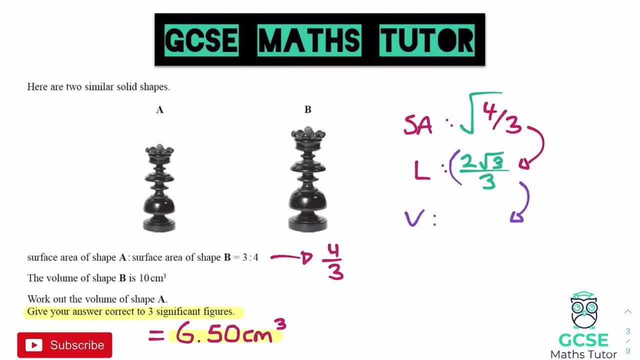 It's going to get quite nasty now. But again, we just need to cube that. So I'll cube the answer. Put that in a bracket. I'm just going to press answer. cubed on the calculator And that gives us a volume scale factor here. 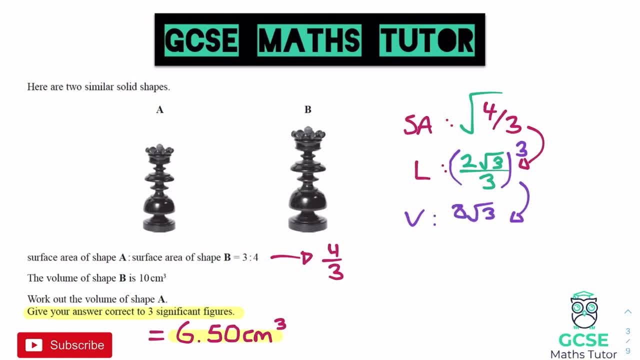 It comes out as 8 root 3 over 9.. And there is our volume scale factor And again we can just use that now to move between the shapes. We are going from shape B down to the smaller shape, So we're going to divide by that scale factor.